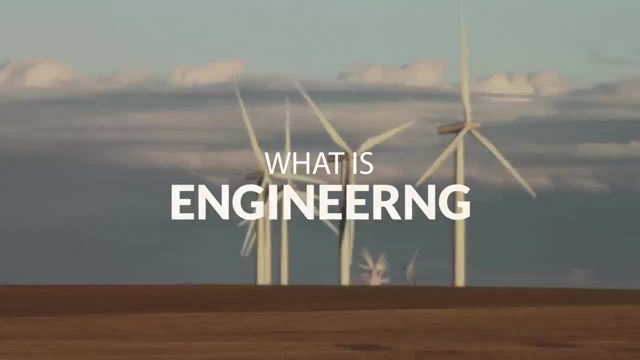 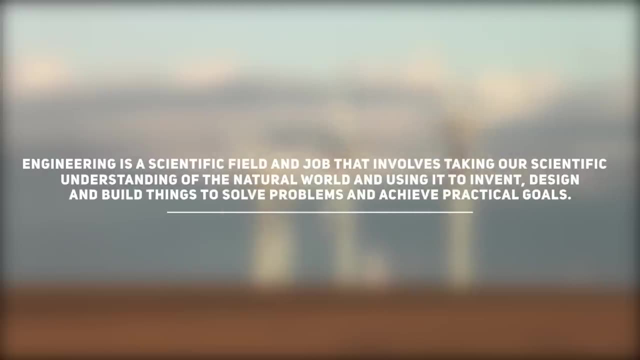 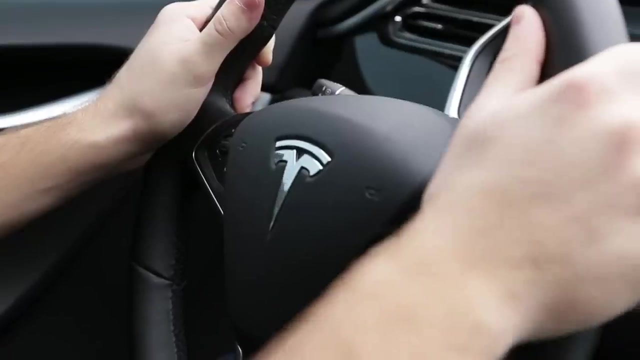 So what is the exact definition of engineering? Well, engineering is a scientific field and job that involves taking our scientific understanding of the natural world and using it to invent, design and build things to solve problems and achieve practical goals. This can include the development of roads, bridges, cars, planes, machines, tools, processes and computers. 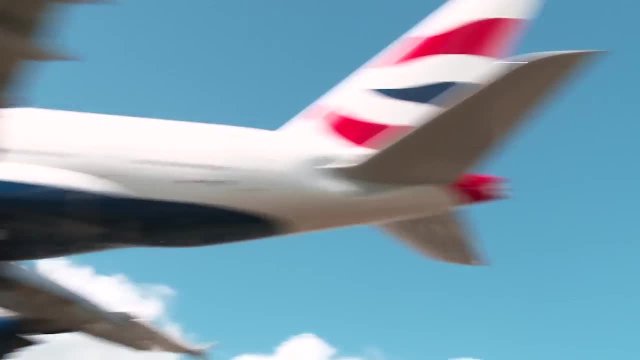 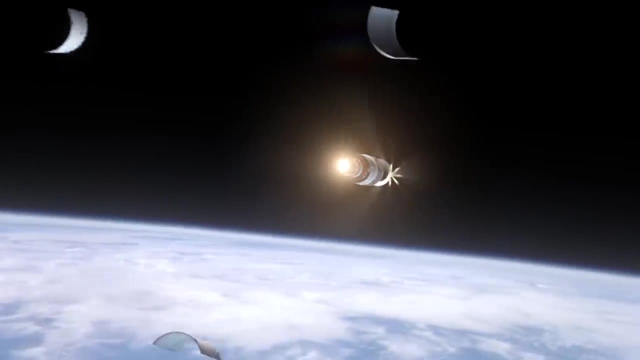 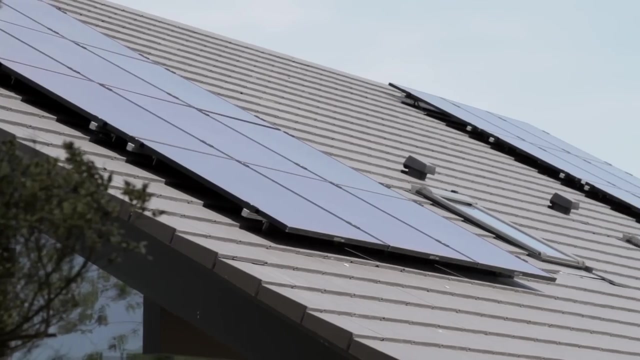 In other words, we can say: engineering is acknowledged as a discipline that opens up opportunities and creates technology and products that help make our lives easier. Engineers are shaping the future by applying their skills to almost everything you can think of, from medicine to renewable energy, food technologies to sustainable mining. 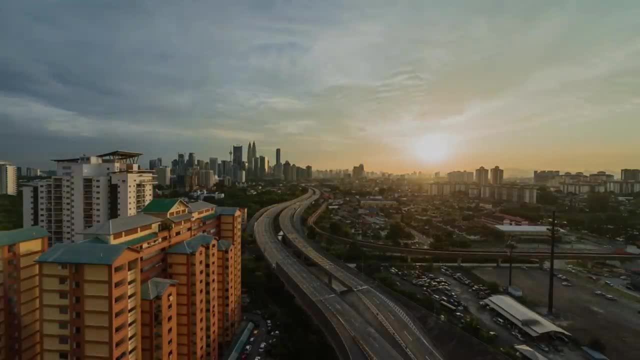 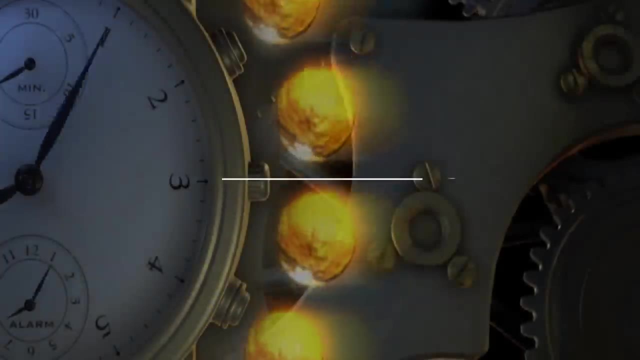 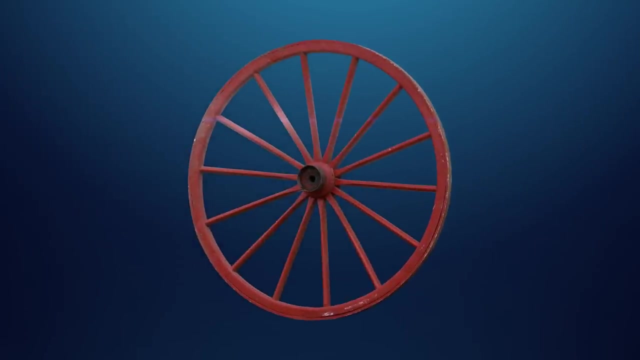 There really is no limit what engineers can do. History of Engineering. The concept of engineering has existed since ancient times, as humans devised fundamental inventions such as the pulley, lever and wheel. Each of these inventions is consistent with the modern definition of engineering. 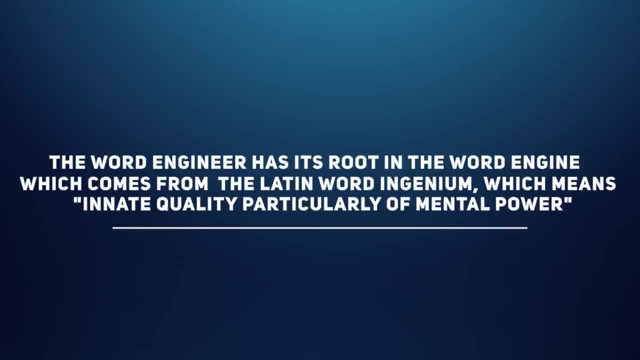 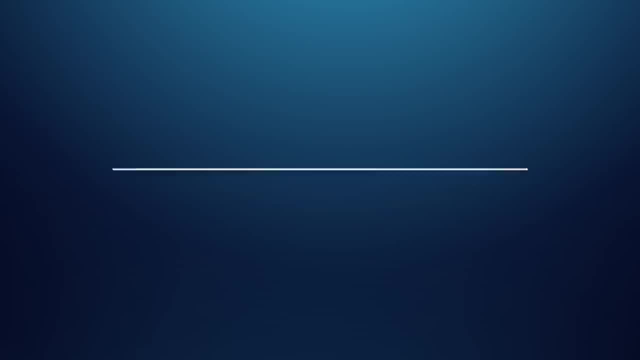 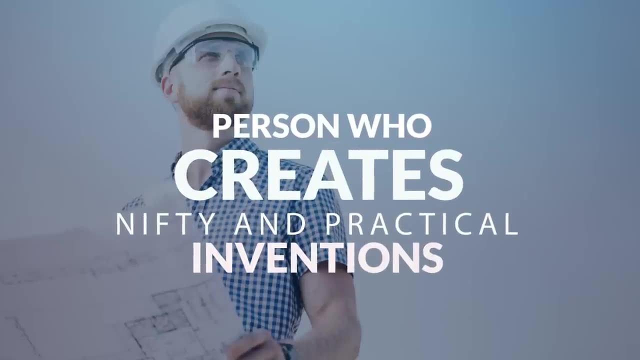 The word engineer has its root in the word engine, which comes from the Latin word ingenium, which means innate quality, particularly of mental power, And thus the word engineer emerged As a person who creates nifty impractical inventions. Branches of Engineering. 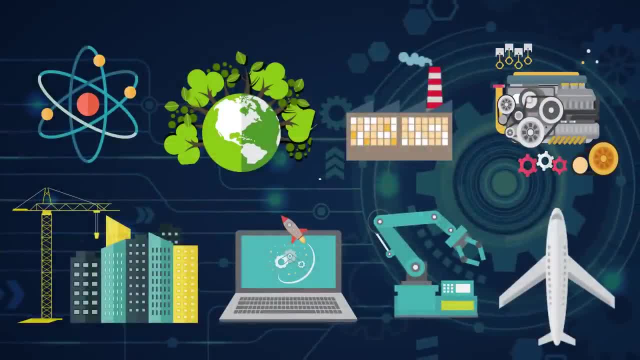 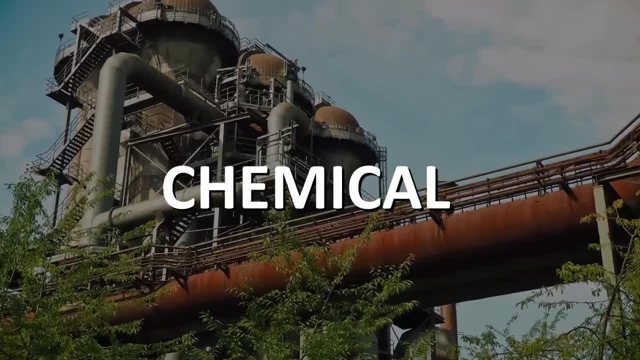 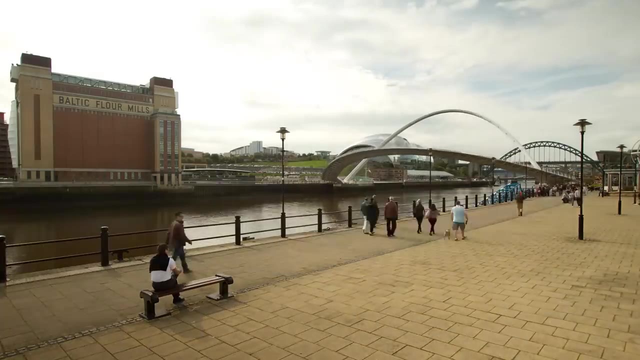 Today, the field of engineering offers more career choices than any other discipline. In the past, there were only four major engineering branches, which include mechanical, chemical, civil and electrical. However, since the human race has been swiftly advancing with regards to technology, 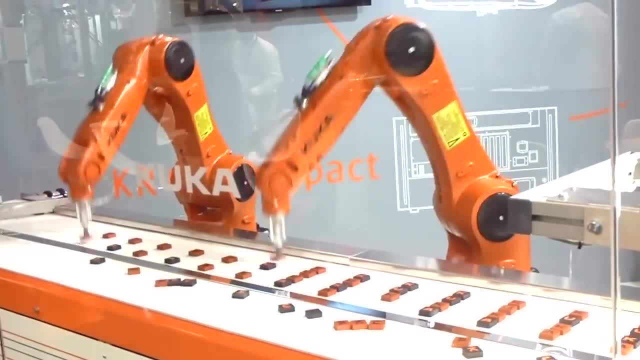 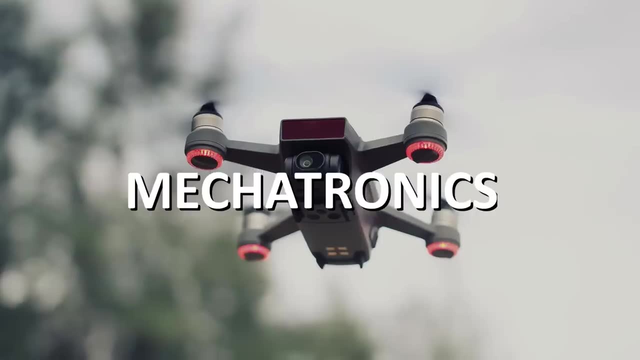 However, since the human race has been swiftly advancing with regards to technology, New branches of engineering are being developed. Engineering jobs can now also be found widely in the computer engineering, software engineering, nanotechnology, mechatronics and many more. What do engineers do? 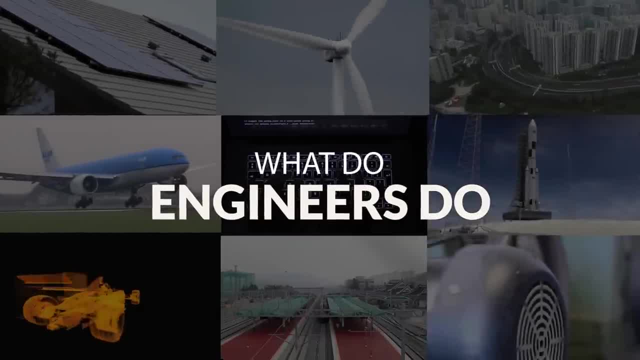 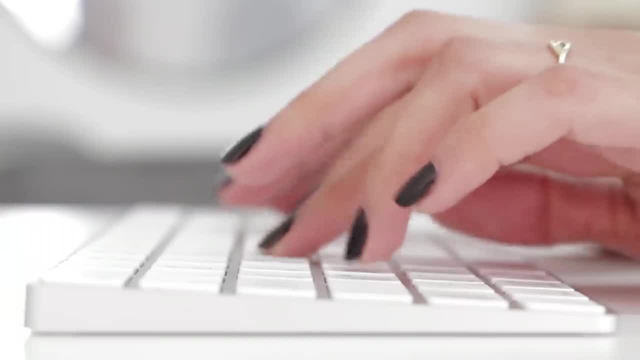 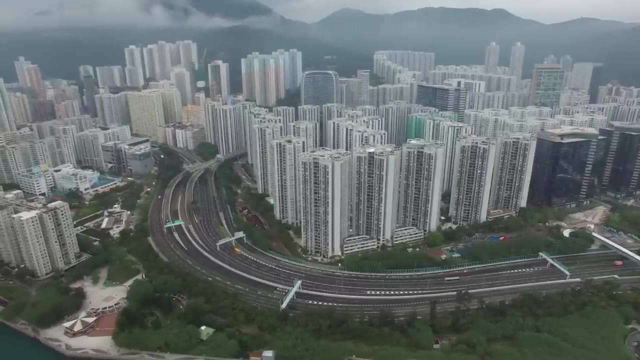 The field of engineering is so vast that it is very hard to define exactly what an engineer does. Yes, engineers still build skyscrapers, design machinery, develop software and oversee public works. But that's only the beginning. They also address society's needs and problems on a number of other scales, with a unique 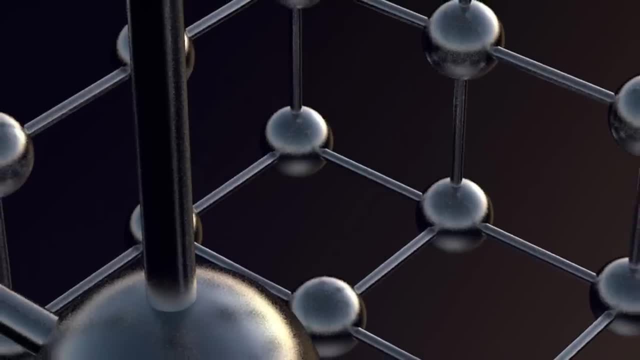 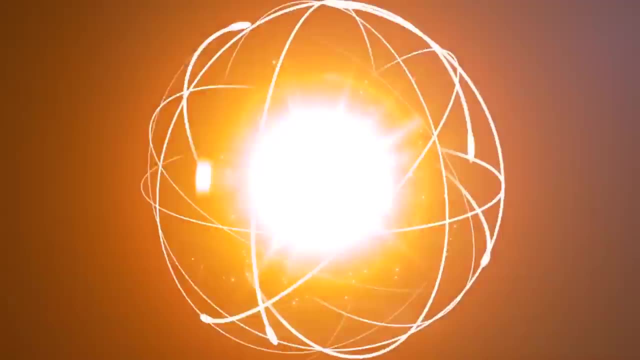 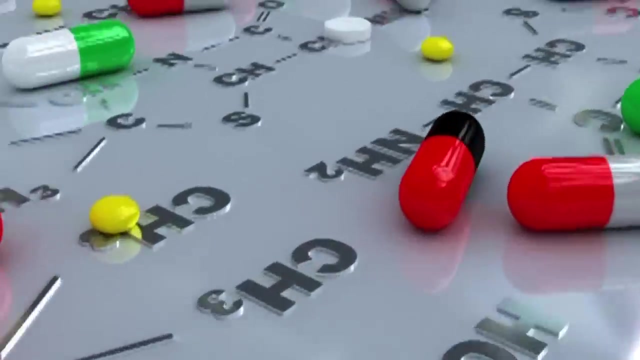 blend of technology and science. At the atomic level, material engineers are developing data storage techniques focusing on the spin of electrons in atoms. At the molecular level, chemical and bioengineers are working on drug delivery systems that work inside cells. At the macro level, environmental engineers are quantifying the particle flow of pollutants. 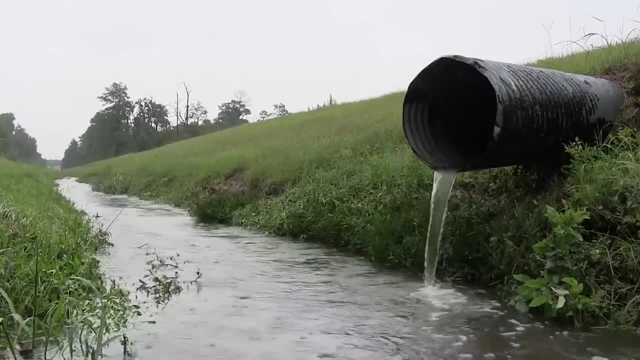 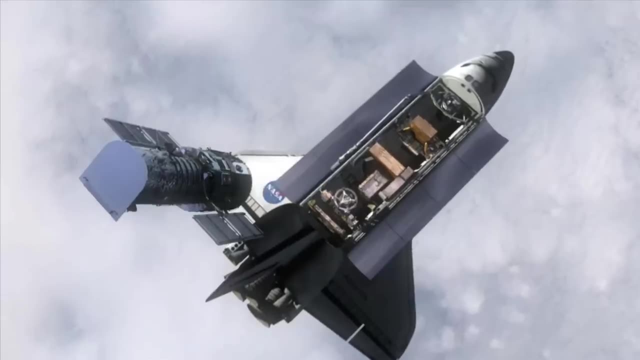 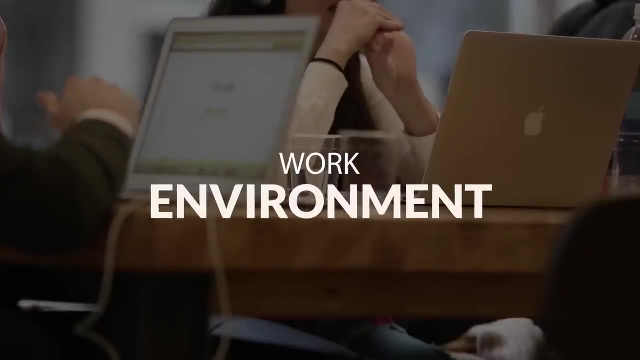 through soil to better understand how to clean up abandoned industrial sites, oil spills and other biohazards. And at the galactic level, astronomical engineers are designing spacecraft for other world exploration Work. Environment: The workplace of an engineer depends on the type of engineer, their actual job description. 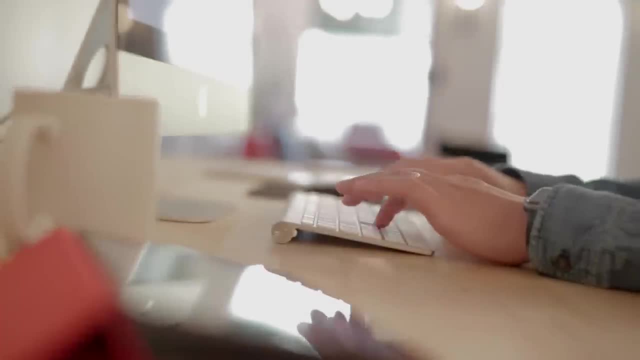 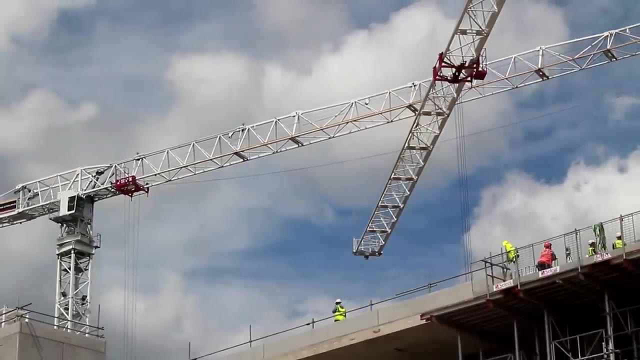 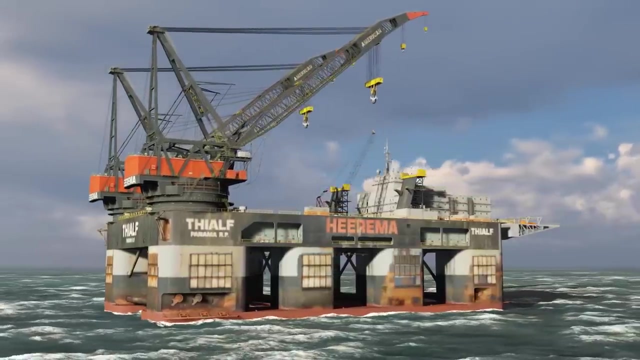 and the company they work for. Many engineers work in an office environment. Some work in industrial plants, Others may spend time outdoors at construction sites And some engineers travel extensively to plants or work sites here and abroad. Many engineers work a standard 40-hour week. 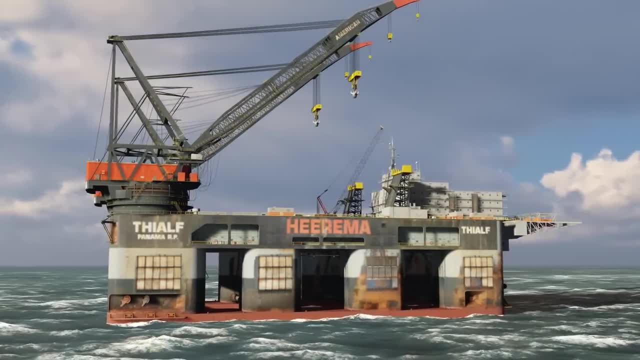 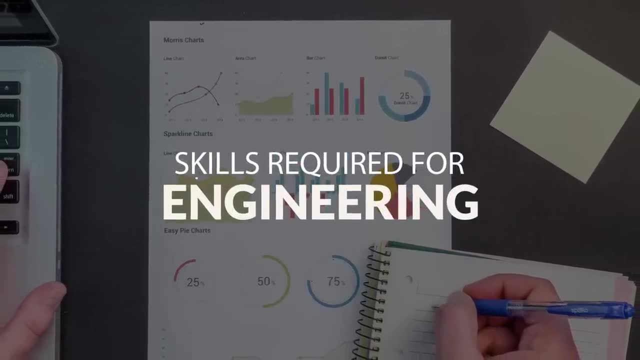 At times, deadlines or design standards may bring extra pressure to a job. Skills Required for Engineering: Most aspiring engineers will need at least a bachelor's degree, more probably a master's degree, from an engineering school. Besides a proper educational background, they may also need a degree in engineering. 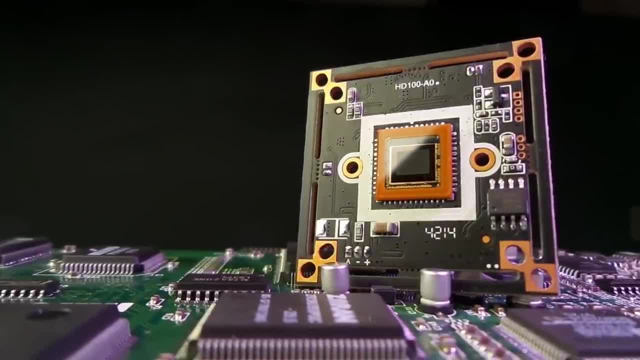 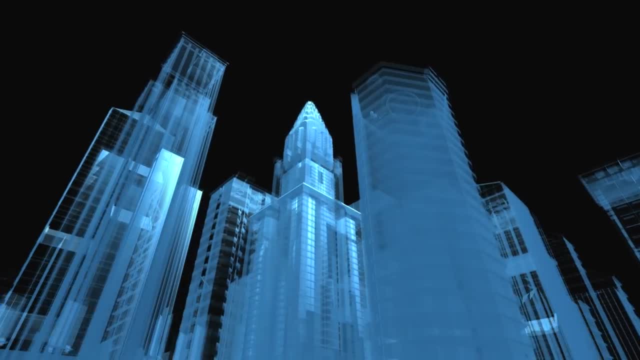 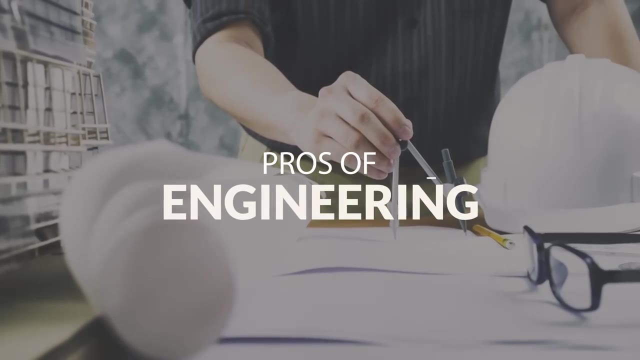 If you have an educational background and relevant technical experience, you will need to demonstrate many soft skills: knowledge of the core subject, application of knowledge, analytical and creative thinking, and familiarity with industry standards. in order to get and keep a good job, Pros of Engineering. Engineering degrees usually dominate the best. 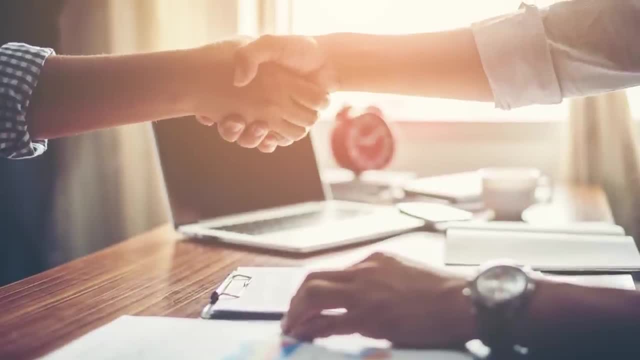 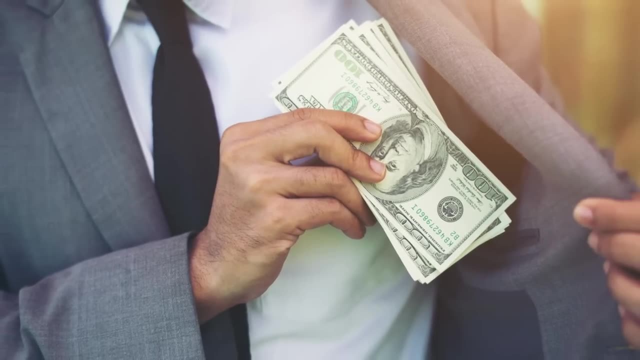 college degrees lists, It's a bit easier to get a job with an engineering degree than with a humanities degree. The best engineering degree is the one with the highest degree. Engineering jobs pay well and are more stable than most other careers. Also, there is a wide variety of job opportunities. 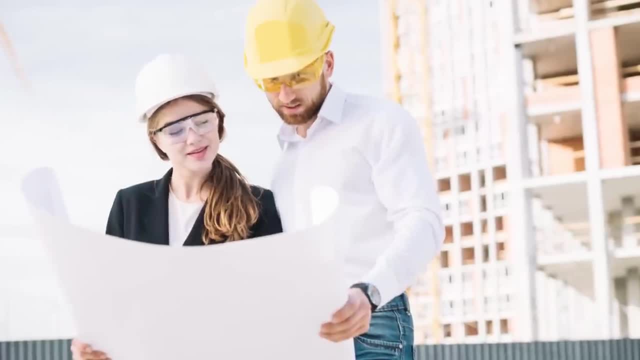 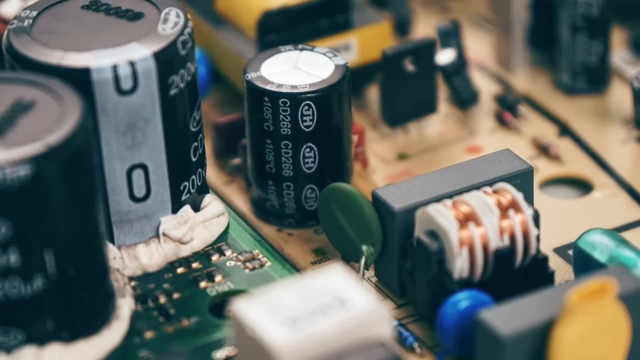 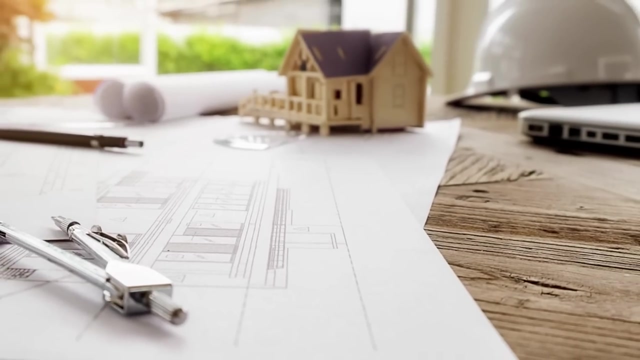 If you like solving problems, then the right engineering job will keep you busily happy. You would finally know how things work in real life. You would finally learn the science or engineering behind all machines. You can design and implement your own creation. Engineers often escalate to management positions and earn extra money.